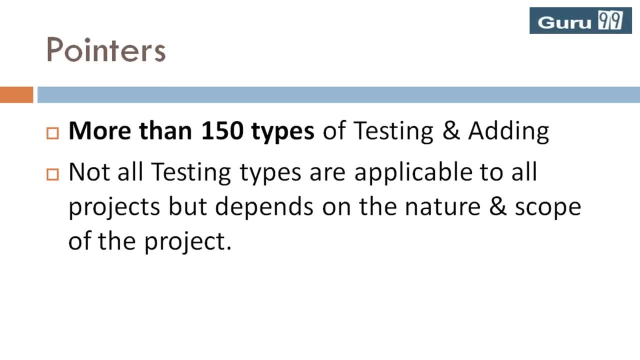 More on this in a later tutorial. Thanks for listening. Subtitles by the Amaraorg community. 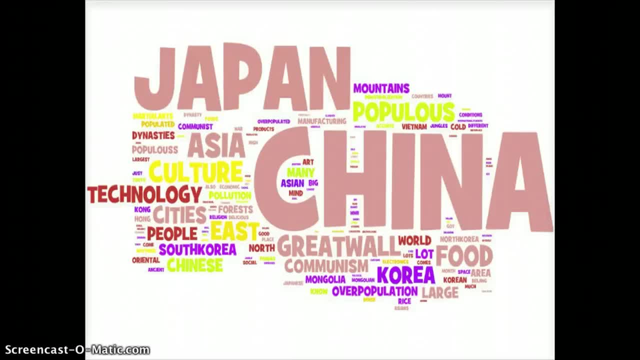 Hello everyone. This week we will be talking about East Asia, So I want to use this lecture to talk a little bit about development in East Asia. I'm going to start with looking at your student impressions of this world region. As you can see, China and Japan loom large in your conceptions of the area. Large populations come up again. You see overpopulated, populous, those sorts of things. 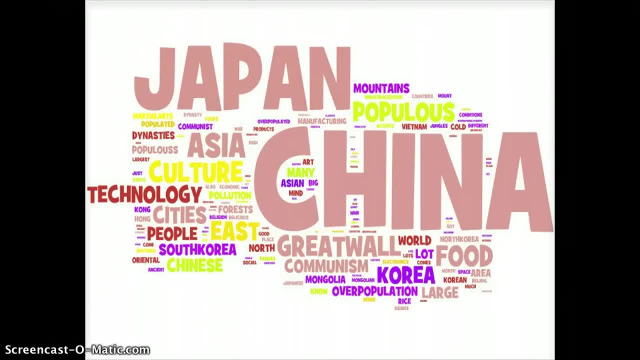 The idea of technology, city and culture. manufacturing is in there as well. So really a lot of ideas about development, for right now We also have this area looming large in the imagination of Americans in terms of understanding development and the shifting of the new international division of labor. 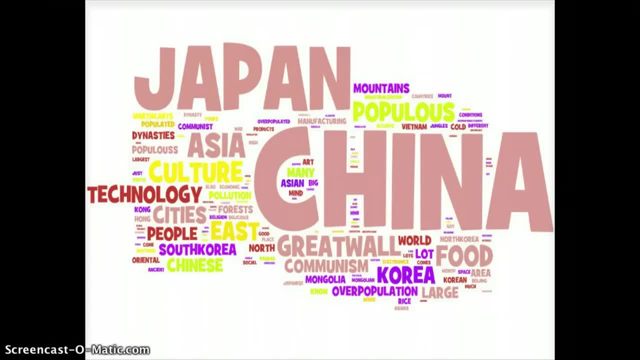 In the last political election, both candidates really took the time to talk tough about China and the perceived loss of American jobs to this part of the world. So we're going to talk a little bit about the developments that led to this new international division of labor and the increase of manufacturing in Japan and China specifically. 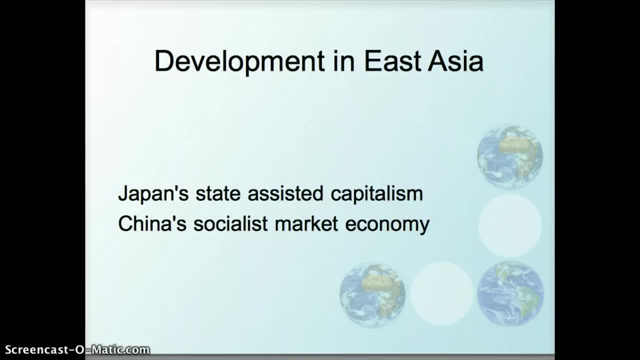 We're going to look at the different countries that these different countries have used for development. In Japan, we have what you can call state-assisted capitalism and in China, a socialist market economy. We're going to look at each one of those things in turn. 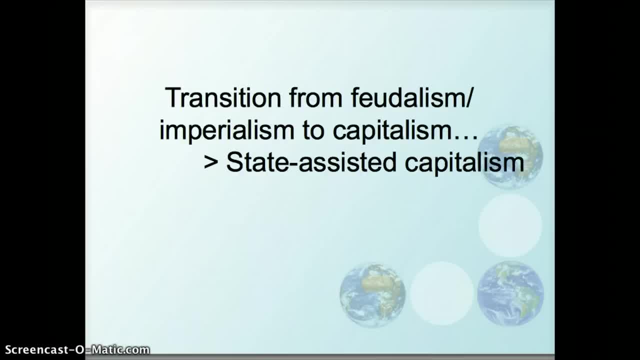 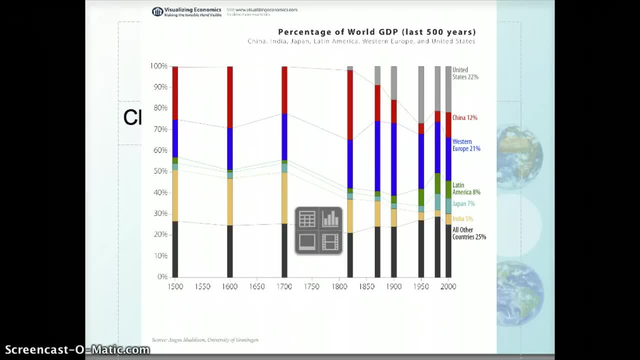